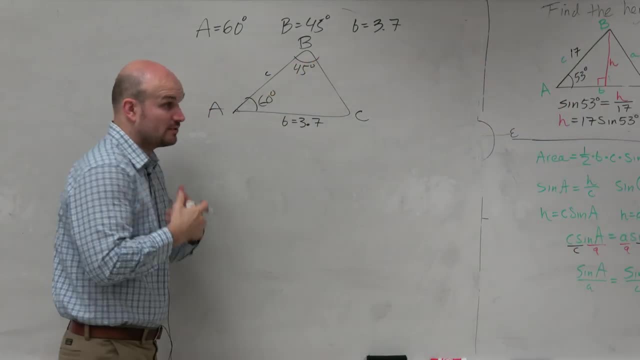 C, we have nothing for. We have nothing for a big C or a little c. So we're going to want to write a proportion. Now again, what I mentioned to you guys before is we want to create a proportion where our unknown is in the numerator. 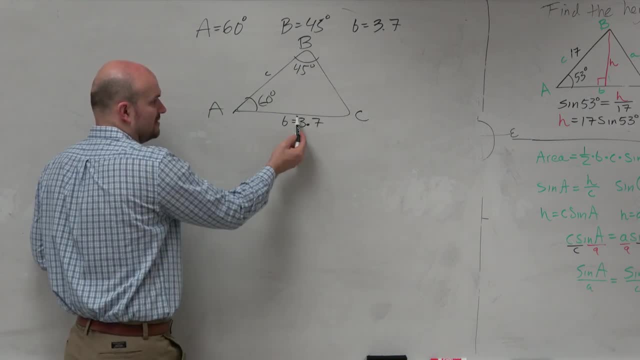 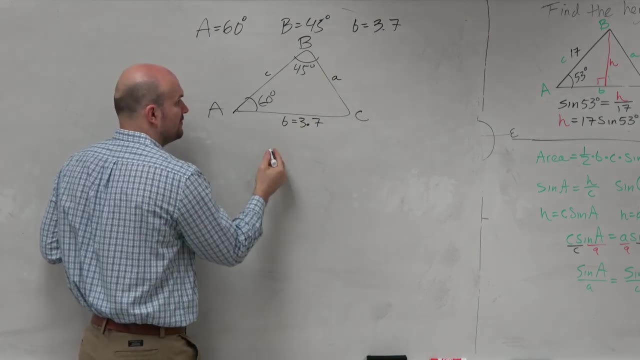 So what do we want to solve for? If we're creating a proportion with this, with angle B and side B, and then we have angle A, that means we're going to want to find side A right. So therefore, I can simply say: 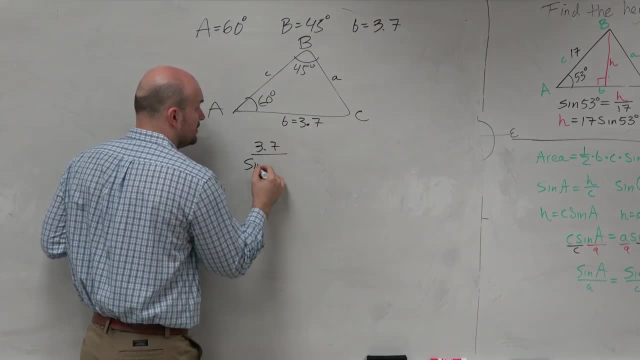 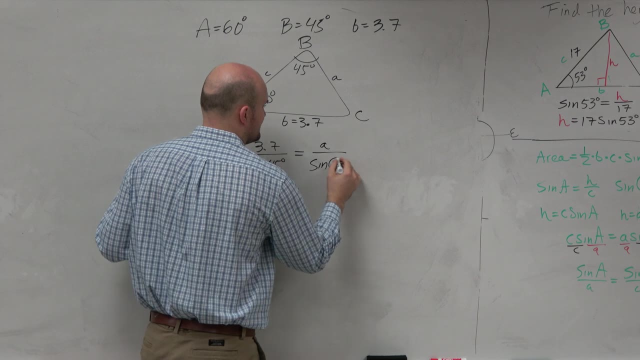 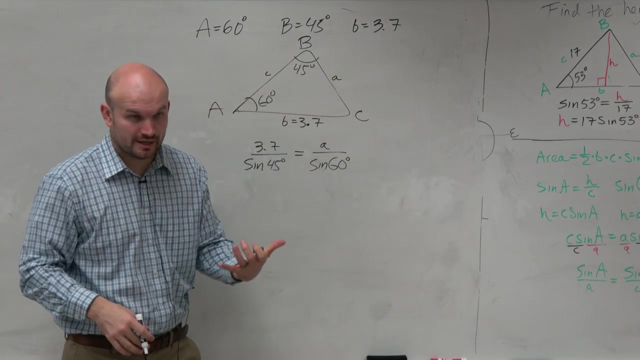 Let's say 3.7 all over the sine of 45 degrees is equal to A over the sine of 60 degrees It can go either way. We always want to have the unknown in the numerator. And again, the reason why this is nice: because this satisfies. 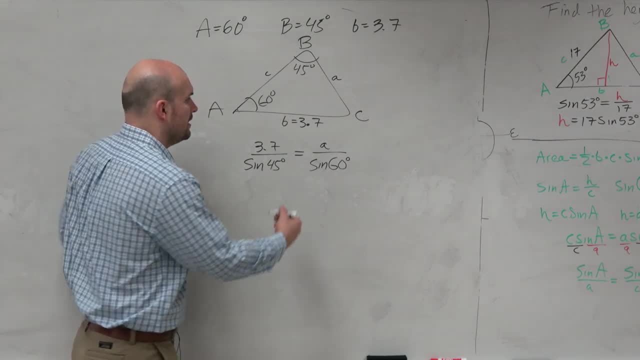 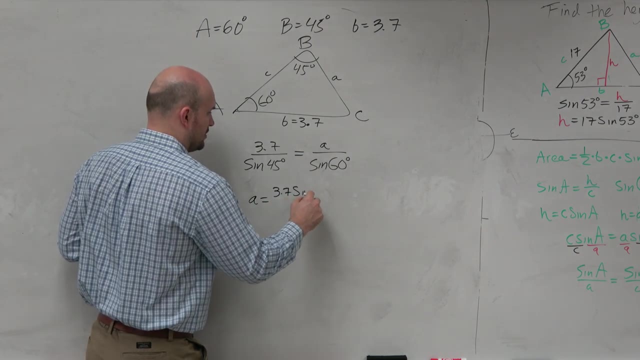 your equation. So if you show this to me, I'm like: OK, good, you showed your equation. I'm just going to show the next step, just for those of you that want to know what to type into your calculator. So all you're doing is multiplying. 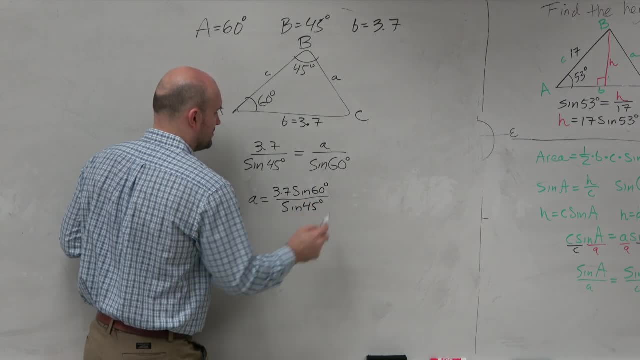 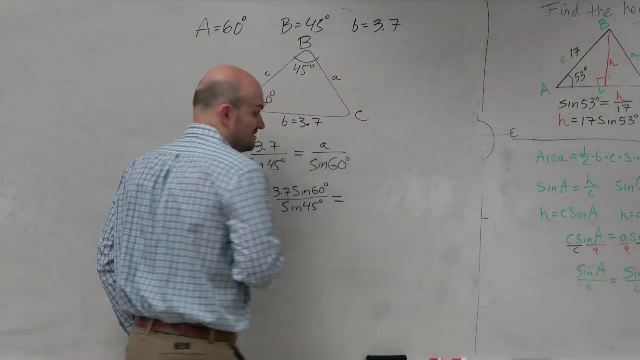 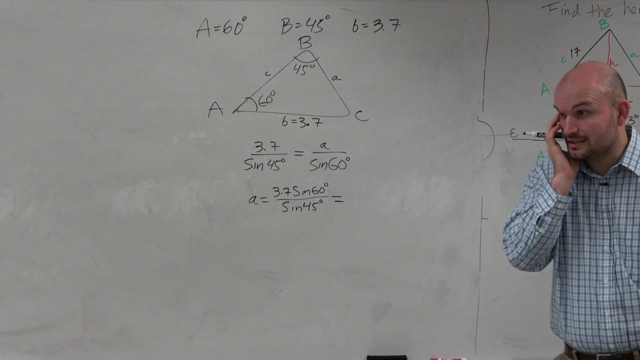 by sine of 60 on both sides, And then you're multiplying by sine of 45 on both sides, And therefore, in that case you get. does anybody do it? I'd love some ambassadors with the calculator. No, no, ambassadors with the calculator. 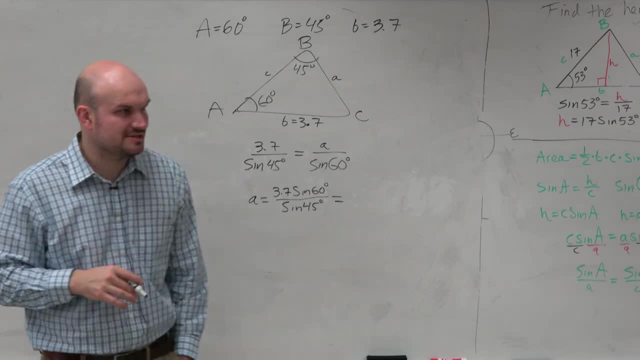 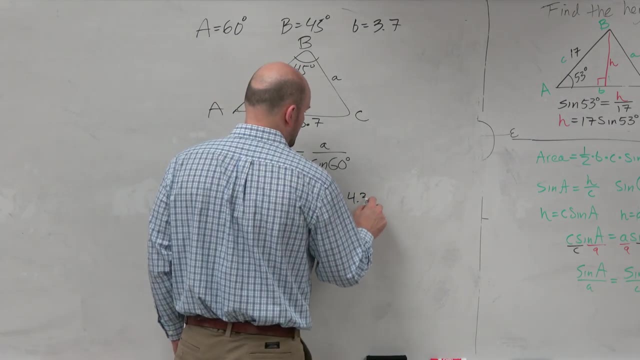 And it's nice. then people let them know and then people make sure that they get the same answer. so we're good. Did you get what? 4.32. 4.32.. Or no? 4.5., 4.532?. 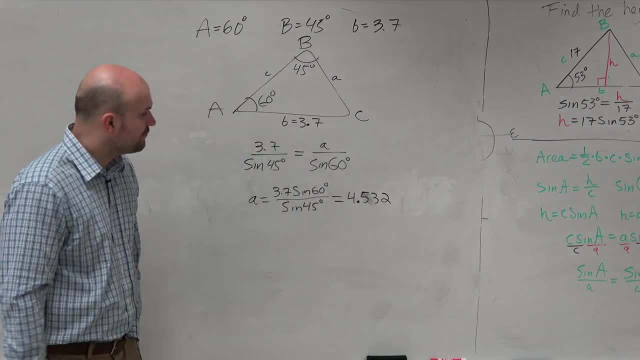 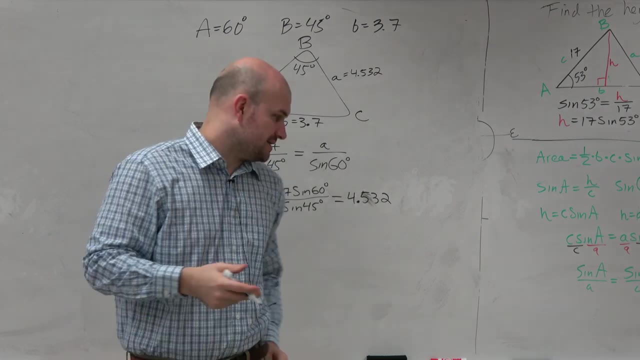 A. Anybody second that? Yes, Yes, OK, So 4.532.. So that is our A Cool All right. Now the problem is: well, actually I'm going to leave this here, I'm just going to get right there. 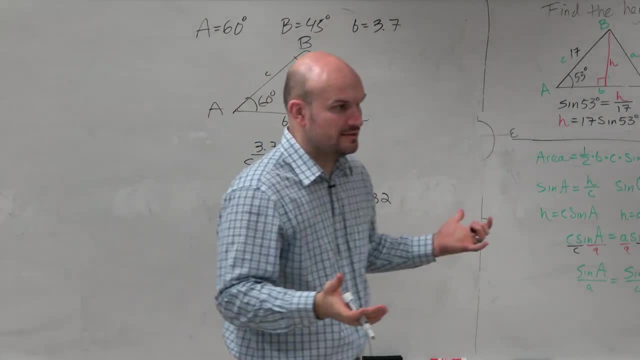 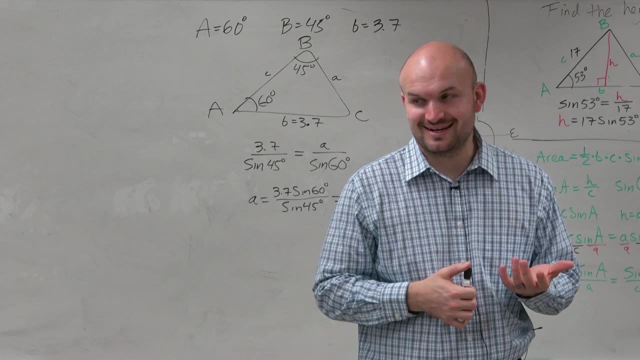 Now the problem is, guys, what do we do about C? We have no information for C. You have the angles. I don't have the angle C though. Well, you have the angles from A to A Right, So what can I do? 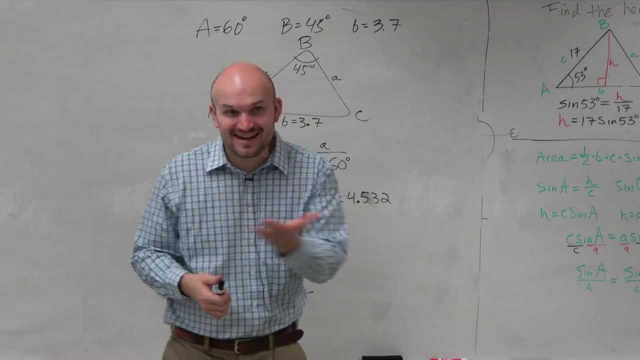 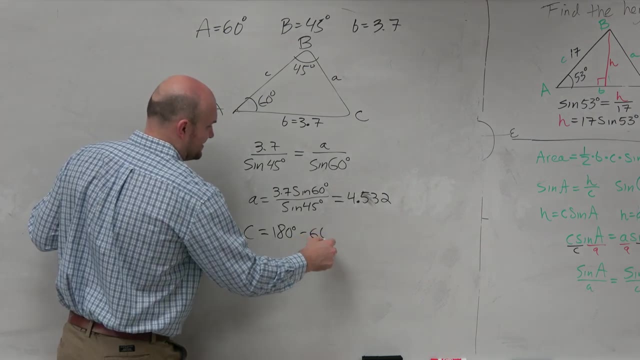 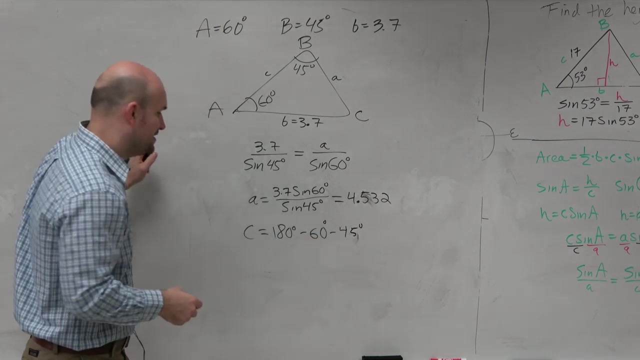 Mind the triangle angle sum theorem. All the angles in a triangle add up to 180? Wow, Awesome. So therefore C is equal to 180 degrees minus 60, minus 45 degrees. I hate that, Right. So therefore this is equal to.